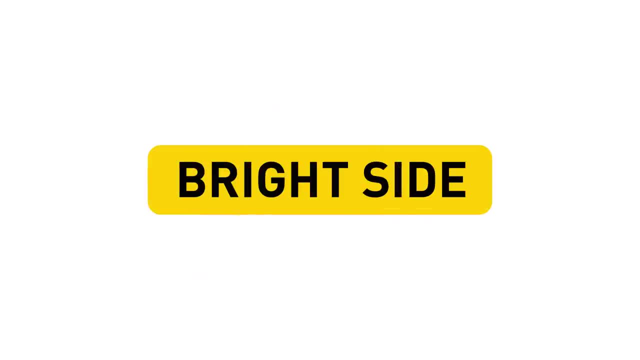 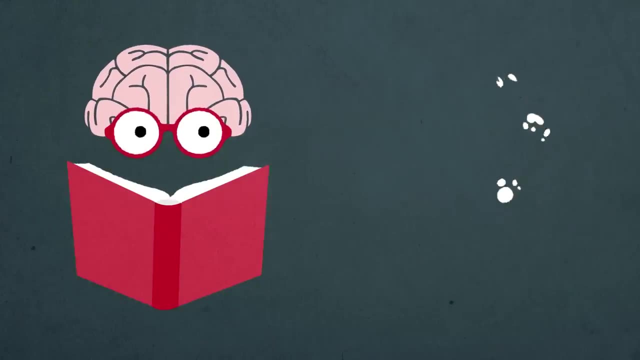 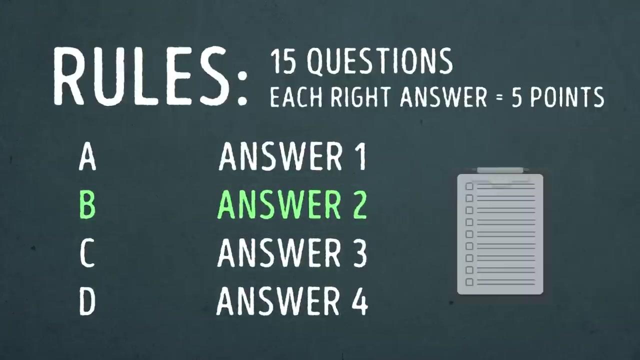 How smart are you for your age? Have you ever wondered how smart you are for your age? Brightside will give you a great chance to find this out. Here are the rules. You will need to answer 15 questions and you will get 5 points for each right answer. Don't forget to count the points, because you will need them to interpret the results at the end of the video. So let's start. 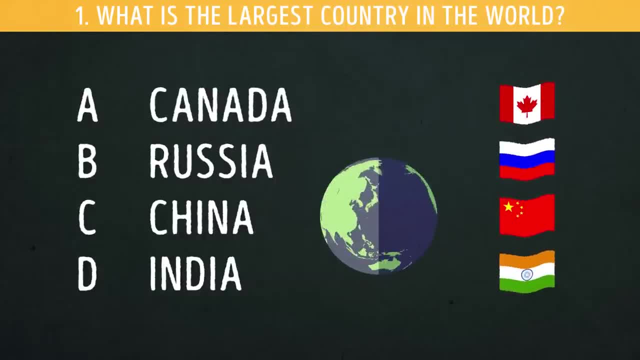 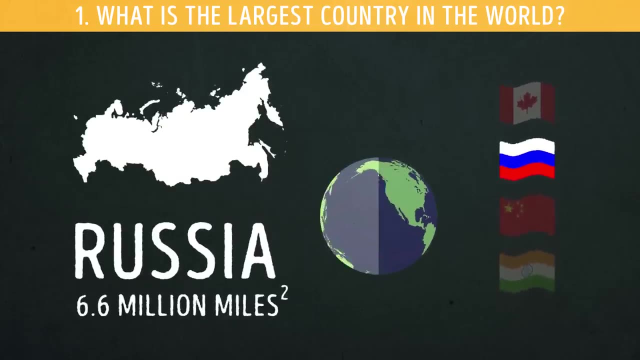 1. Let's start with something simple: What is the largest country in the world? A- Canada, B- Russia, C- China, D- India. And the right answer is Russia. It covers 6.6 million square miles- So much space. 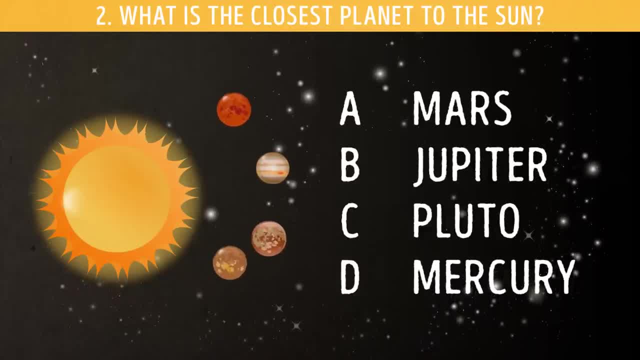 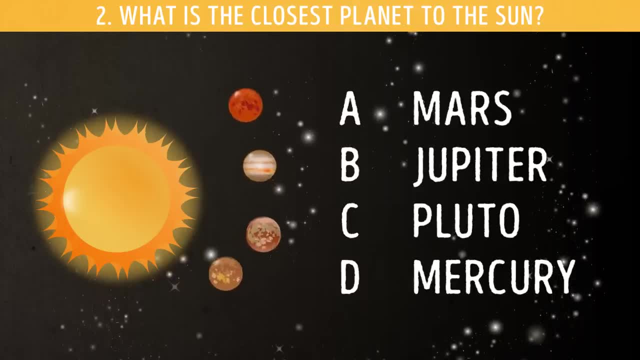 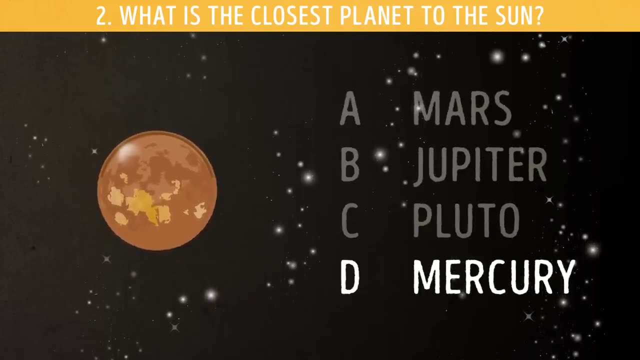 2. What is the closest planet to the Sun? A- Mars, B- Jupiter, C- Pluto, D- Mercury. Of course it's Mercury. A year on Mercury is just 88 days. By the way, as of 2006,, Pluto is not a planet anymore. The definition of the planet was changed and poor Pluto failed to fit the description. 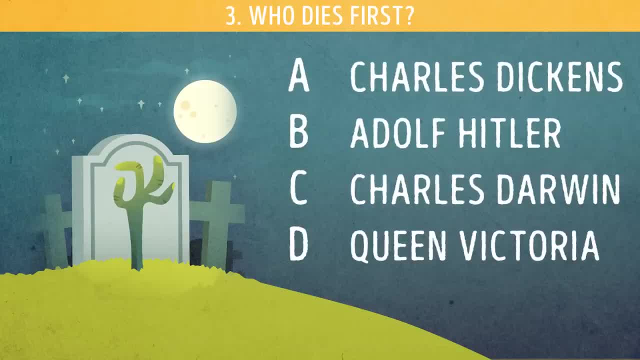 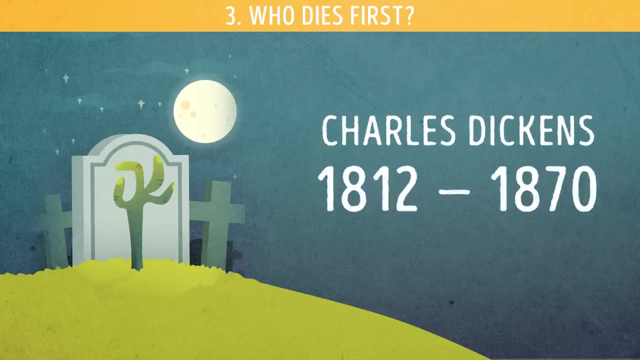 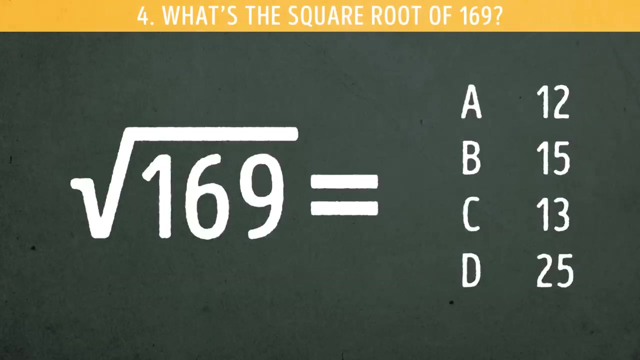 Now how about some history? 3. Who dies first? A- Charles Dickens, B- Adolf Hitler, C- Charles Darwin, D- Queen Victoria. Charles Dickens was the first to die. 4. What's the square root of 169?? A, 12. B, 15. C, 13. D, 25.. 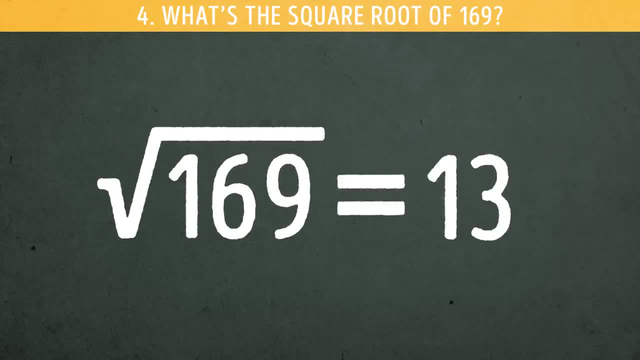 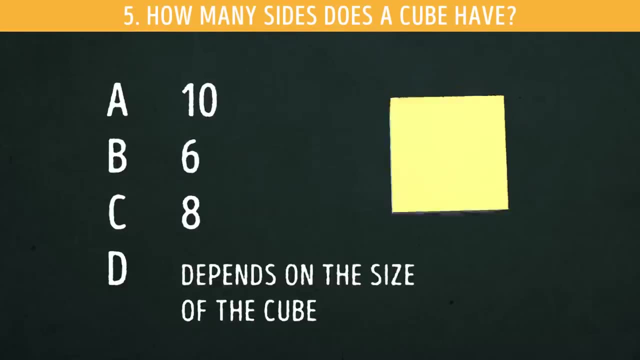 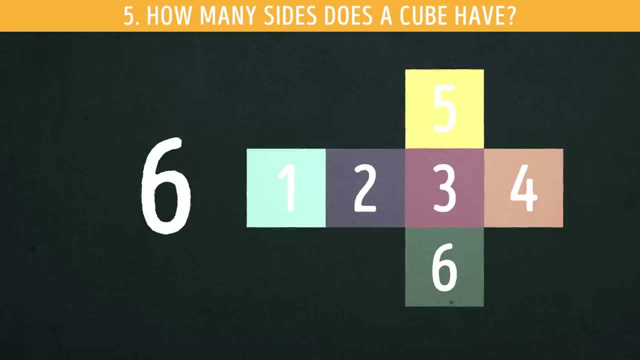 Well, this one is pretty easy: It's 13. 5.. How many sides does a cube have? A, 10. B, 6. C, 8. D Depends on the size of the cube. Of course, it doesn't depend on the size of the cube. It has six sides, no matter what. 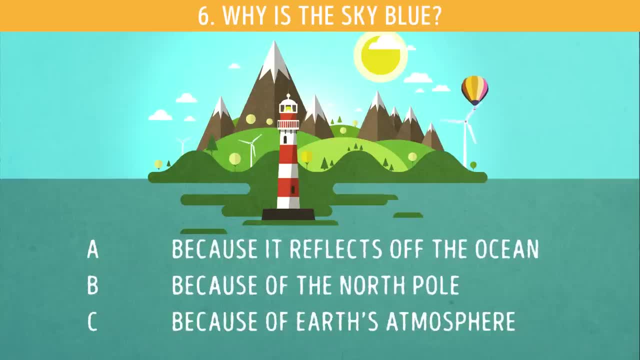 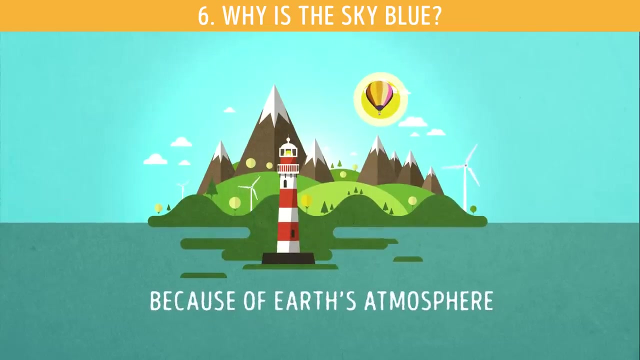 6. Why is the sky blue? A- Because it reflects off the ocean. B- Because of the North Pole. C- Because of Earth's atmosphere. The right answer is C. The thing is. light that comes from the Sun scatters in the atmosphere of our planet. Shorter waves scatter more. That's why all we have left from a visible light is the blue color. 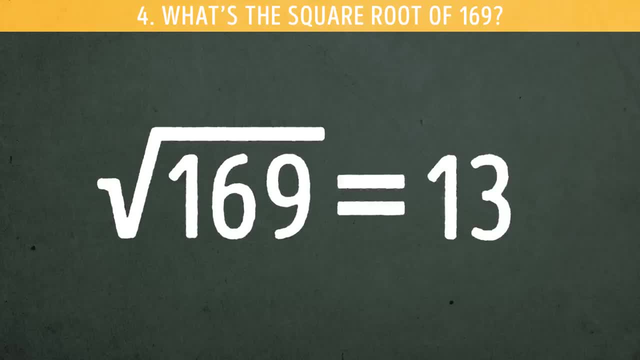 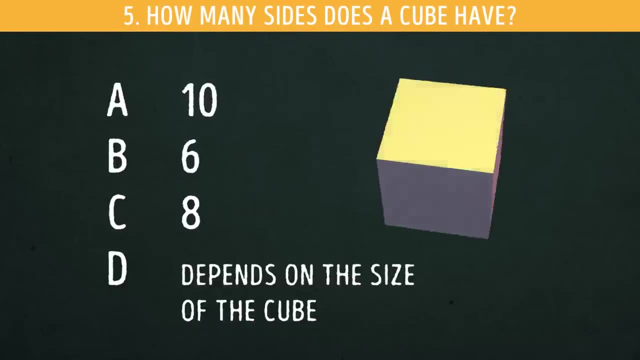 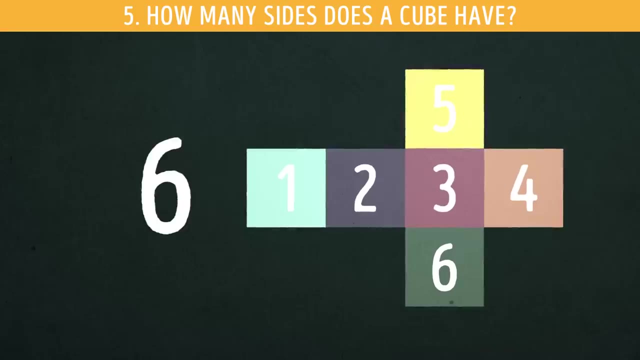 Well, this one is pretty easy: It's 13. 5.. How many sides does a cube have? A, 10. B, 6. C, 8. D Depends on the size of the cube. Of course, it doesn't depend on the size of the cube. It has six sides, no matter what. 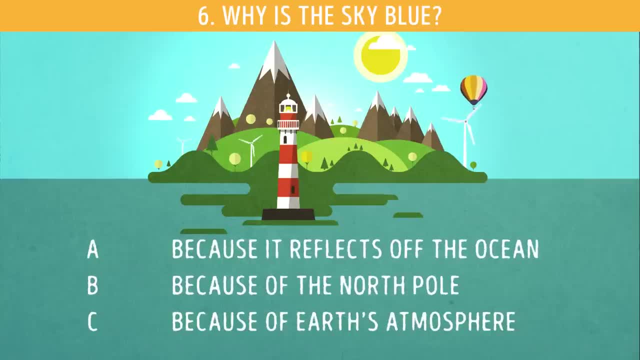 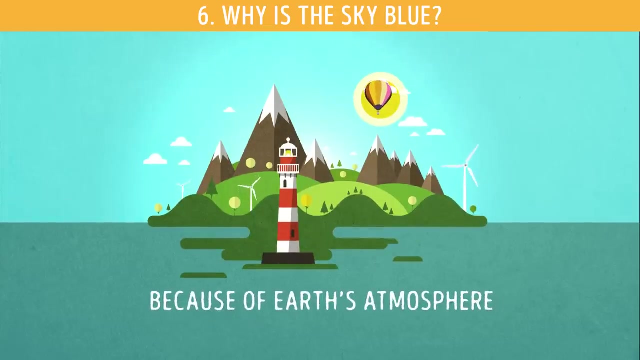 6. Why is the sky blue? A- Because it reflects off the ocean. B- Because of the North Pole. C- Because of Earth's atmosphere. The right answer is C. The thing is. light that comes from the Sun scatters in the atmosphere of our planet. Shorter waves scatter more. That's why all we have left from a visible light is the blue color. 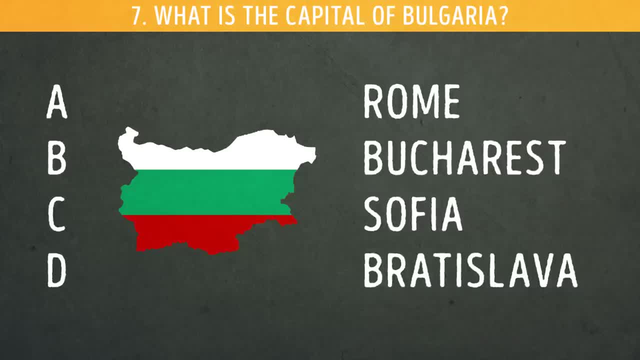 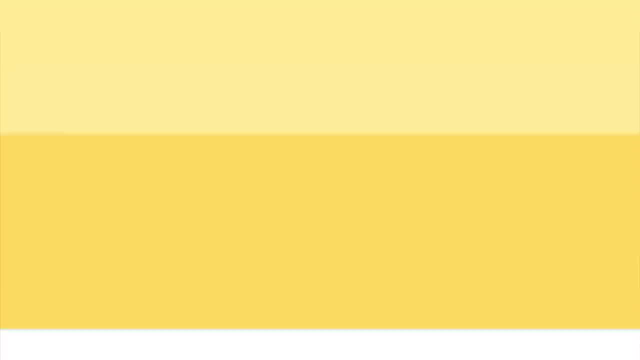 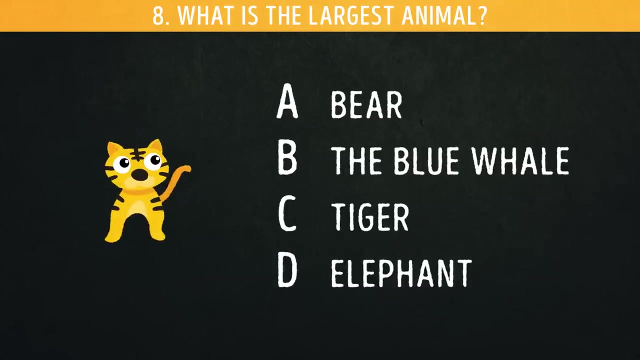 7. What is the capital of Bulgaria? A- Rome, B- Bucharest, C- Sofia, D- Bratislava. Alright, it's Sofia. Let's go to the next question. 8. What is the largest animal? A- Bear, B- The blue whale, C- Tiger, D- Elephant. 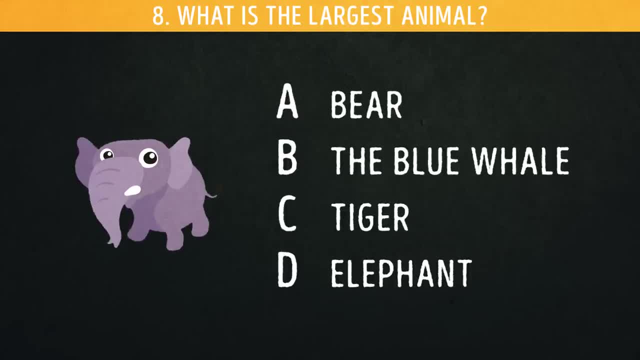 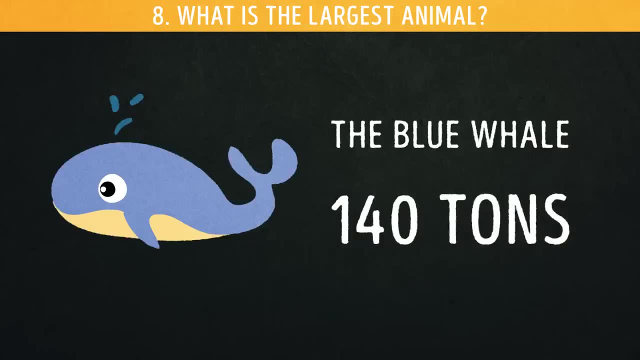 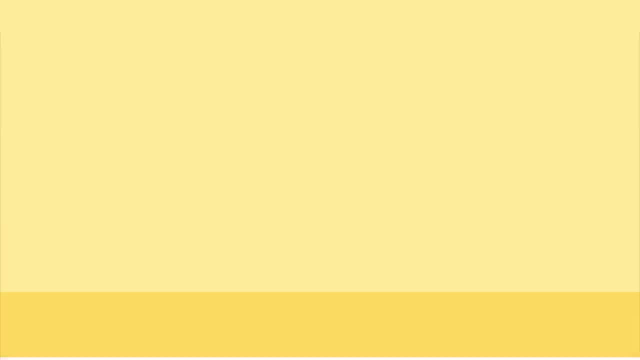 The largest animal is the blue whale. it can be as big as 140 tons. can you even imagine such a giant thing? by the way, you can watch a great video on our channel about ten cute animals that can actually kill you. number nine: who wrote the catcher in the 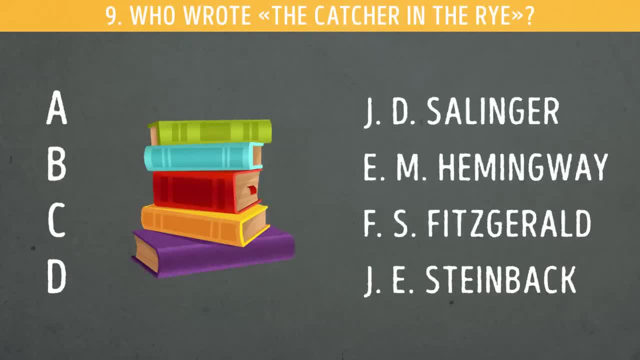 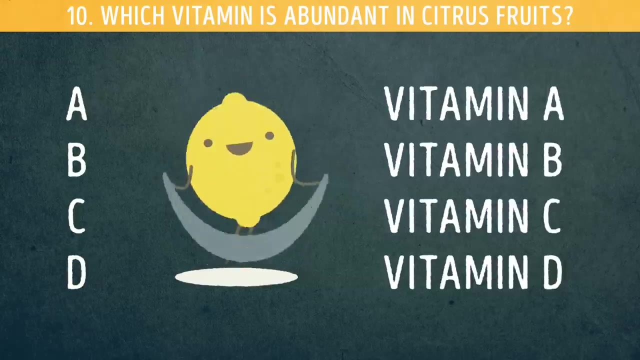 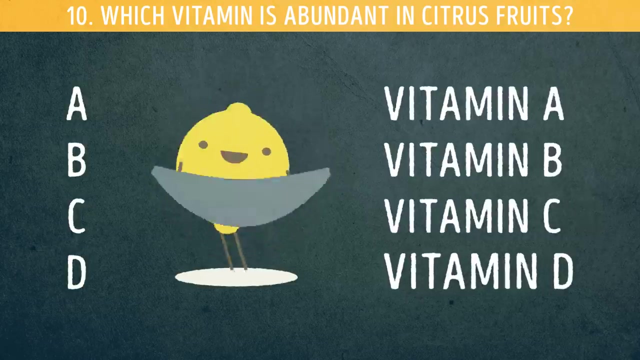 ride a JD Salinger, be EM Hemingway. see FS Fitzgerald. DJ a Steinbeck. this book was written by JD Salinger. everyone should know this stuff. 10: which vitamin is abundant in citrus fruits? a vitamin a, B, vitamin B, C, vitamin C, D, vitamin D you. 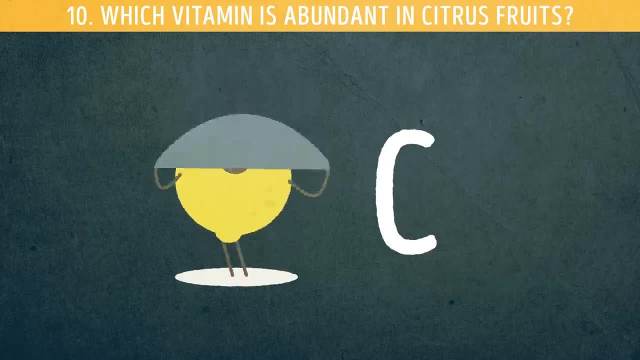 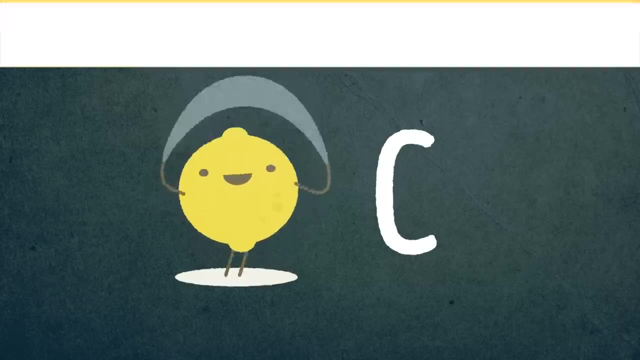 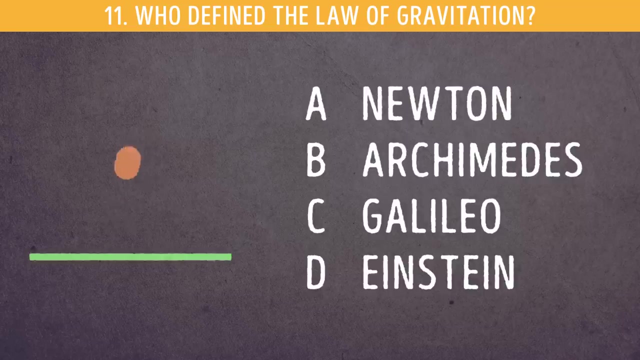 know, see citrus easy to memorize. doctors say that when you are sick, you should eat oranges, because they have a lot of vitamin C and it helps you to recover faster. 11: who defined the law of gravity? a. Newton, B. Archimedes, C. Galileo, D. Einstein. the right answer is Newton. you. 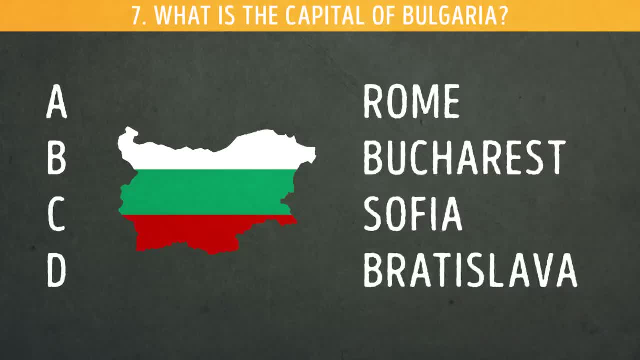 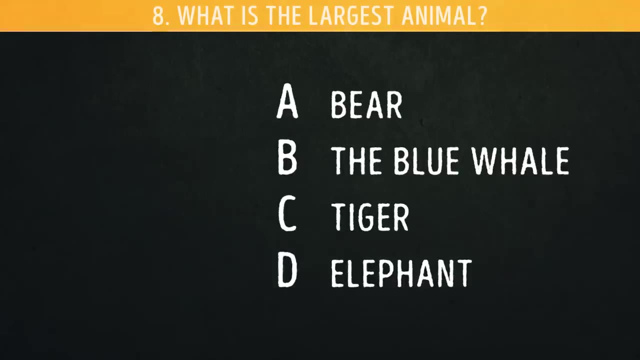 7. What is the capital of Bulgaria? A- Rome, B- Bucharest, C- Sofia, D- Bratislava. Alright, it's Sofia. Let's go to the next question. 8. What is the largest animal? A- Bear, B- The blue whale, C- Tiger, D- Elephant. 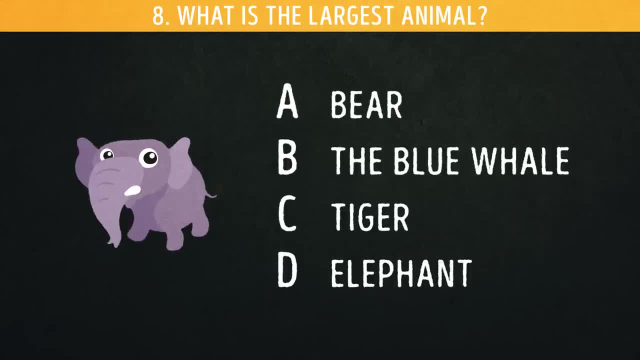 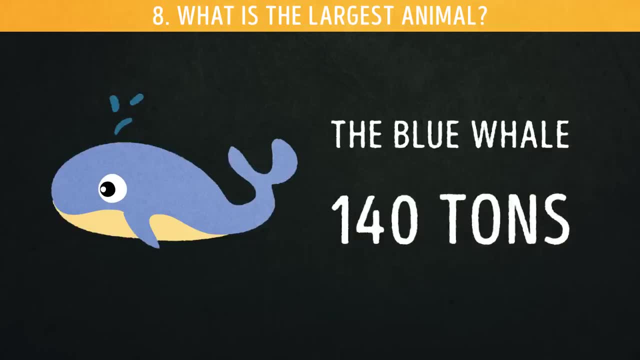 The largest animal in the world is the blue whale. It can be as big as 140 tons. Can you even imagine such a giant thing? By the way, you can watch a great video on our channel about 10 cute animals that can actually kill you. 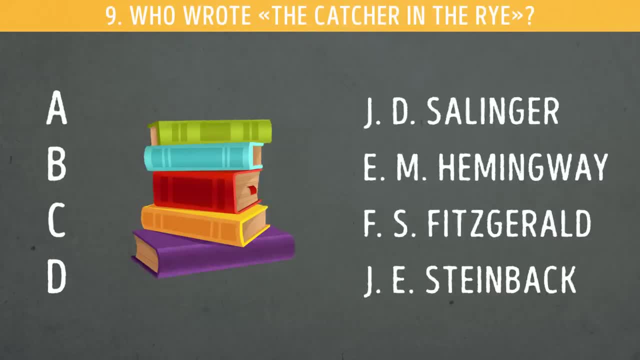 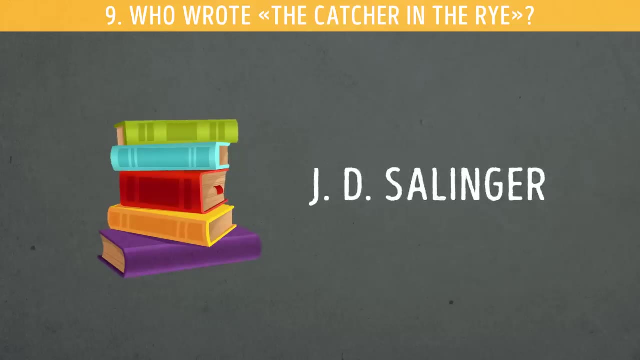 9. Who wrote The Catcher in the Rye? A J D Salinger, B E M Hemingway, C, F S Fitzgerald, D, J A Steinbeck. This book was written by J D Salinger. Everyone should know this stuff. 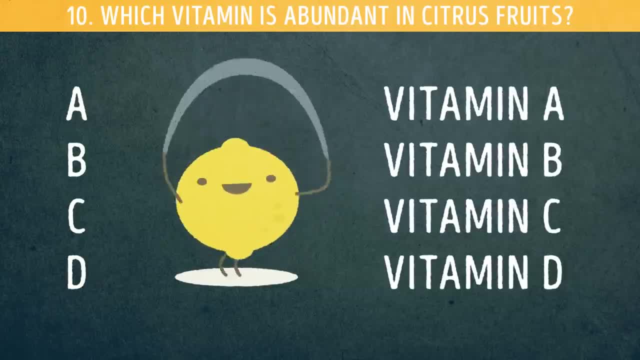 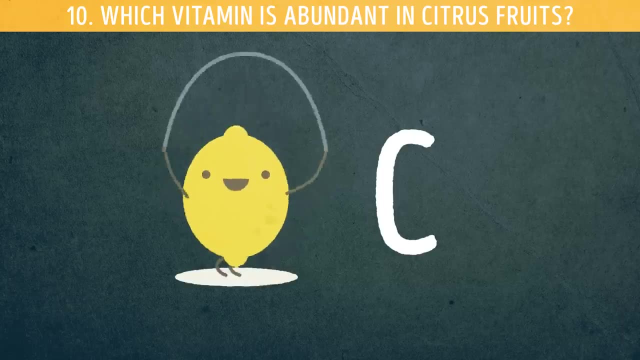 10. Which vitamin is abundant in citrus fruits? A, Vitamin A, B, Vitamin B, C, Vitamin C, D, Vitamin D? You know C Citrus, Easy to memorize. Doctors say that when you are sick you should eat oranges, because they have a lot of vitamin C and it helps you to recover faster. 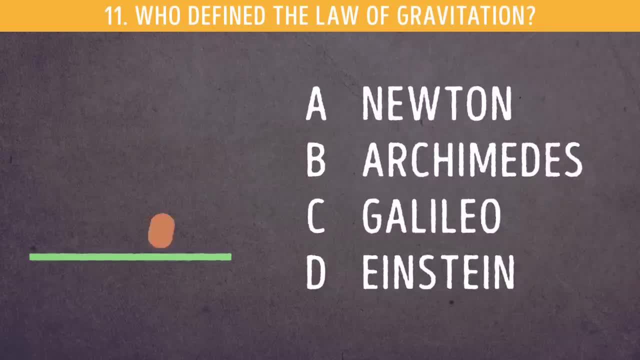 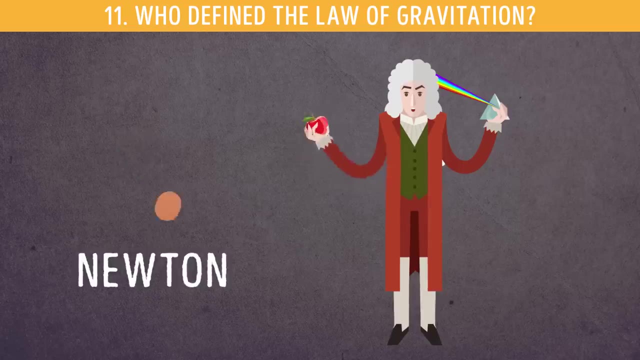 11. Who defined the law of gravitation? A Newton, B Archimedes, C- Galileo, D- Einstein. The right answer is Newton. You probably know the story about an apple falling on his head. We're not sure if the story is true, but Newton was definitely the first one who defined the law of gravitation. 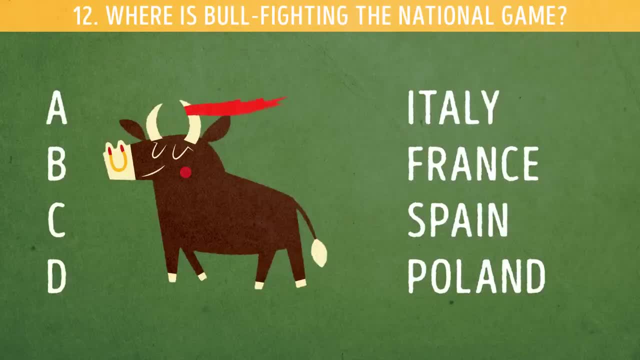 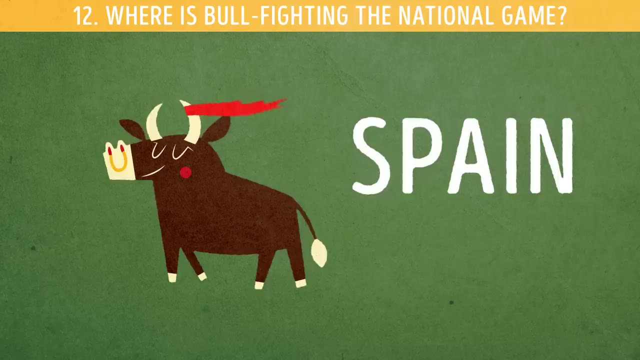 12. Where is bullfighting the national game? A- Italy, B- France, C- Spain, D- Poland. Bullfighting, or corrida, is the national game in Spain. However, as of 2010,, bullfighting was banned in Catalonia, but not yet in the rest of Spain. 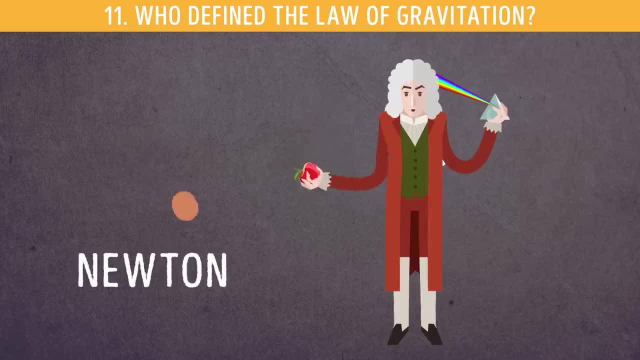 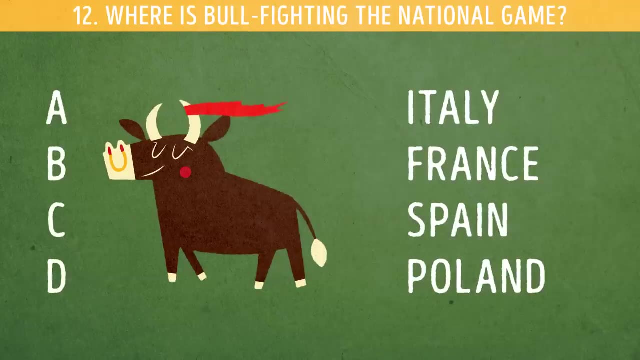 probably know the story about an apple falling on his head. we're not sure if the story is true, but Newton was definitely the first one who defined the law of gravitation. 12: where is bullfighting? the national game? a- Italy, B, France, C, Spain, D- Poland. 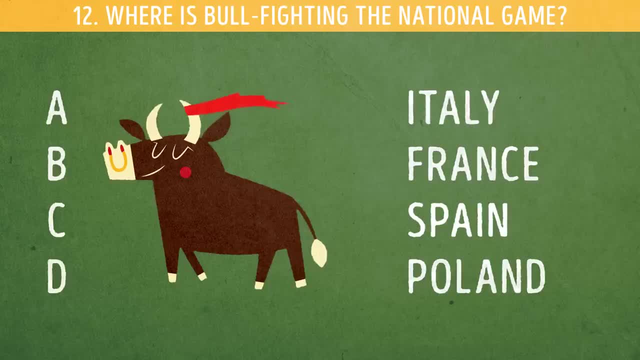 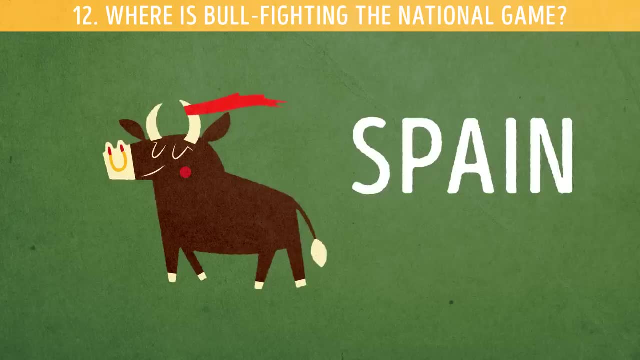 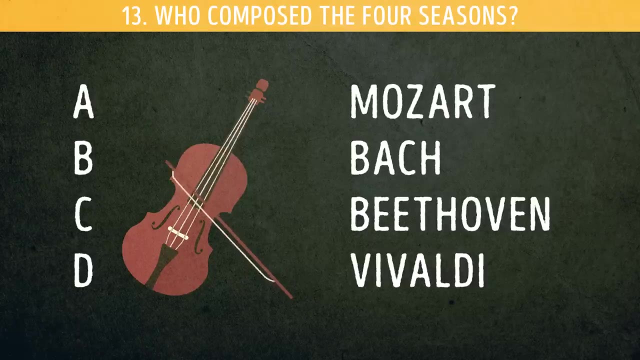 bullfighting, or corrida, is the national game in Spain. however, as of 2010, bullfighting was banned in Catalonia, but not yet in the rest of Spain. 13 who composed the Four Seasons: a, Mozart, B, Bach, C, Beethoven, D, Vivaldi, the Four. 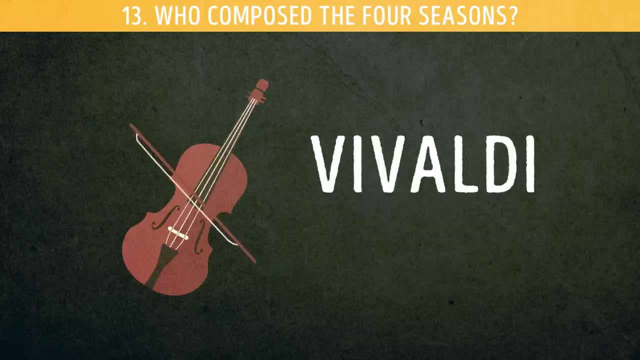 Seasons, which is a beautiful piece of music, was composed by Antonio Vivaldi. 14. who defined the law of gravity? B, Bach, C, Beethoven, D Vivaldi. the Four Seasons, which is a beautiful piece of music, was composed by Antonio Vivaldi. 15. what is the name of the device that is used to see objects on the surface? 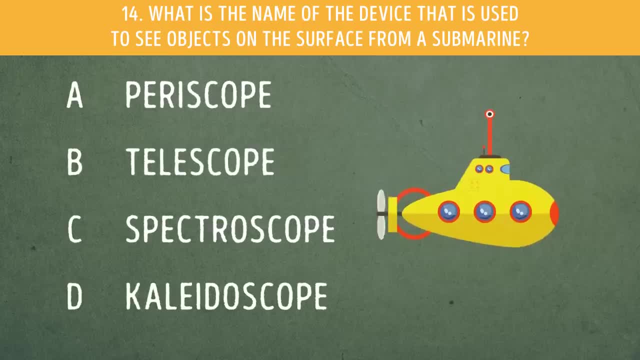 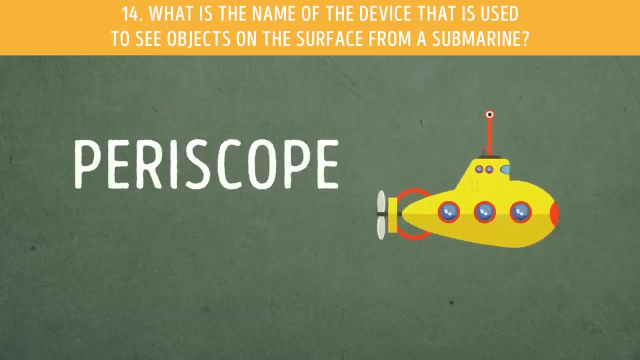 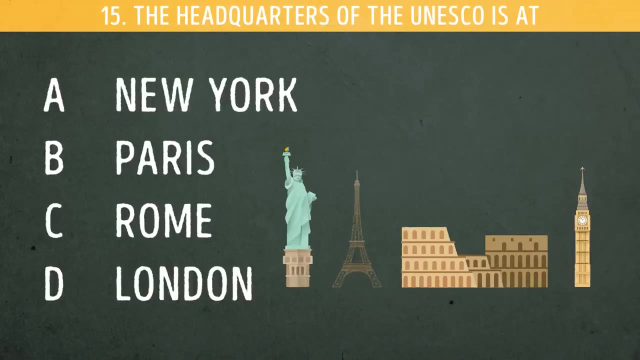 from a submarine, a periscope, B telescope, C spectroscope, D kaleidoscope? the right answer is periscope. and now for the last question, 15. the headquarters of the UNESCO is at a New York, B Paris, C Rome, D London. this organization is situated in. 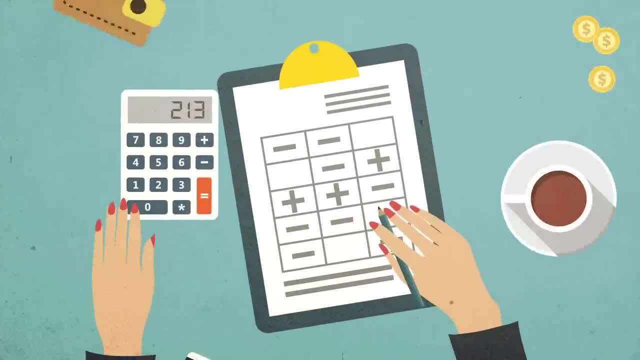 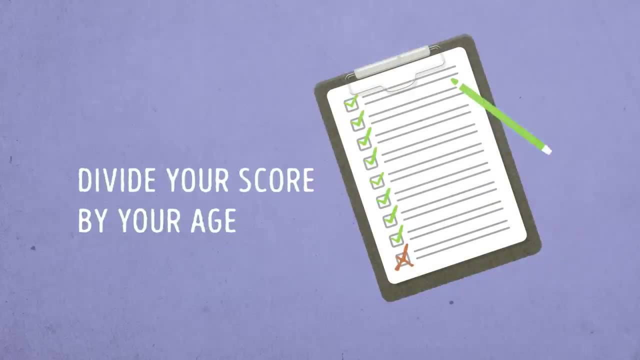 Paris, France. now it's time to calculate the results. you get five points for each right answer. now enter your score into the calculator and divided by your age. but if you are younger than 10, divided by 10, and if you are older than 18, divide your. 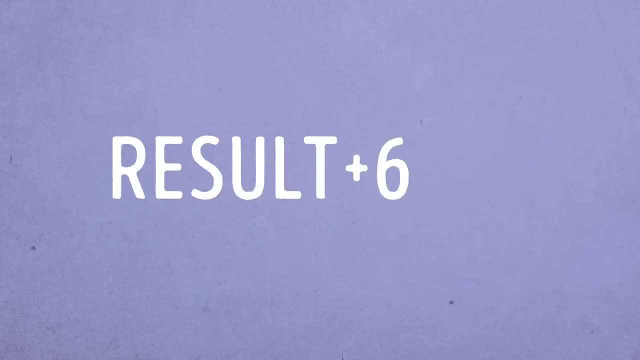 score by 18. now, when you have a number, add six to it and let's check what your score means. you are extremely smart. you have a great general knowledge. congratulations. you are intelligent enough for your age. this is a good result. it means you should read more books and learn harder to improve your 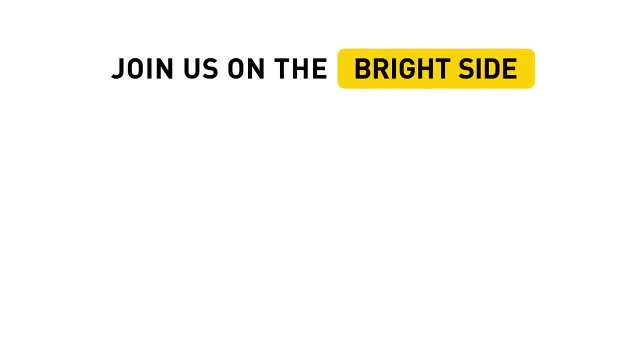 general knowledge. are you satisfied with your result? tell us in the comment section below. don't forget to like this video and send it to your friends to compare your results with them and, of course, click Subscribe to join us on the bright side of life.